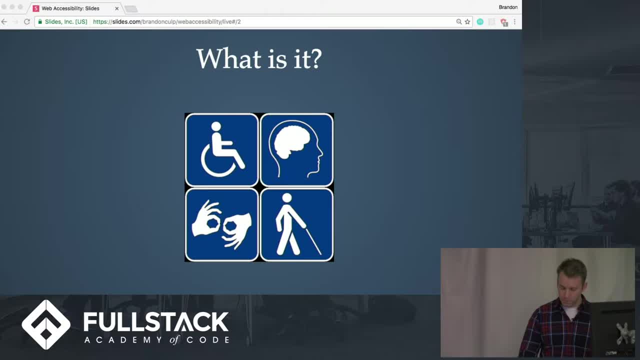 just have the main different types of disabilities. So we have a physical disability, so someone that was, you know, born without a limb or maybe has a temporary injury or develops arthritis throughout their life. We have a cognitive disability, so someone that maybe has difficulty. 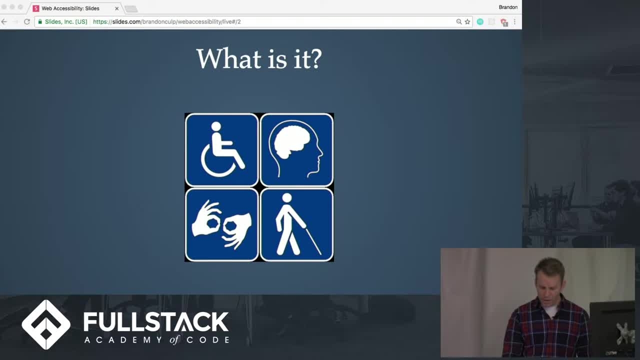 reading or spelling, And then we have a hearing impairment. So you know someone that's hard of hearing, as well as someone with visual impairment, So either someone that's colorblind or completely blind. So some of the tools these people might use to access the web. 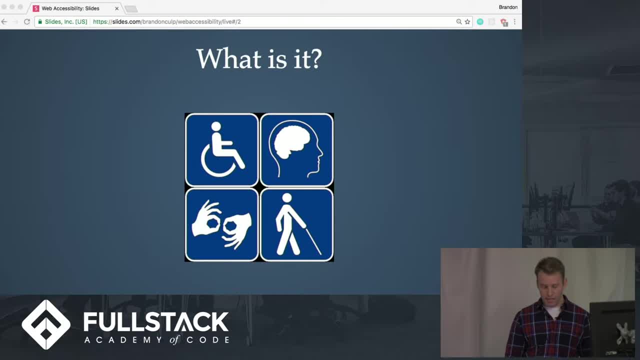 So for a physical disability, maybe like speech to text, cognitive like text to speech, or error correction. software for hearing like closed captioning or a, basically a transcript of a video, And then, for someone with a visual impairment, a screen reader or a browser that allows you. 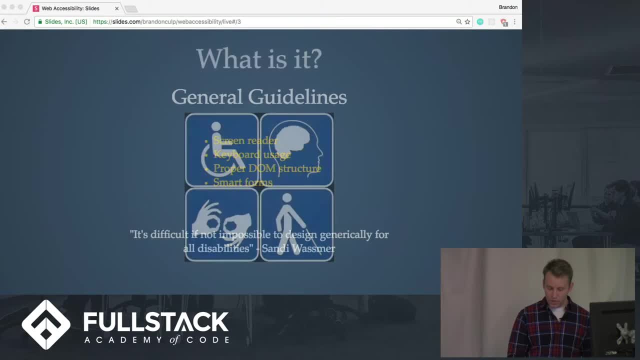 to use your keyboard instead of a mouse. So some general guidelines to keep in mind when you're thinking about your own websites and making them accessible. So can your site be accessed using a screen reader? So one of the big things here is having alternative. 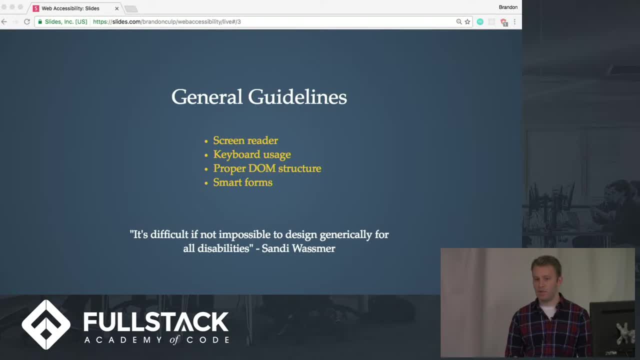 text for images and giving your links unique and descriptive names. Can you use a keyboard to access things You know? is it solely clicking, Or can you just use a keyboard to move around the site? Is your DOM properly set up? So do you have, like, the proper semantic structure? So are. 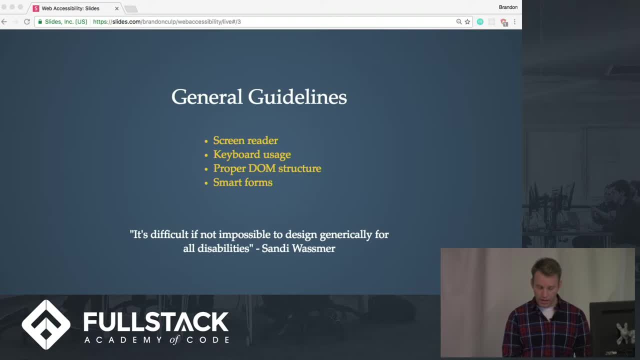 your headings set up right, Can you access the site in high contrast mode. And then my favorite, smart form. So can you fill out the forms you know, not only using a keyboard, but can you also use your voice to fill them out, And I like this quote down here at the: 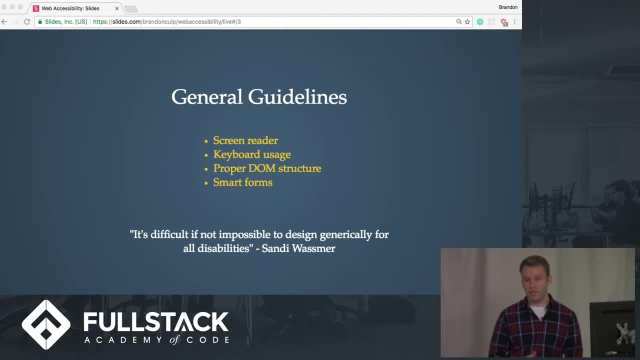 bottom. Basically just something to keep in mind. If you think about accessibility, there's really no way to make your site completely accessible to every single person out there, So it's a good idea to just think about your target audience and focus on a couple disabilities. So our focus today is going to be on physical 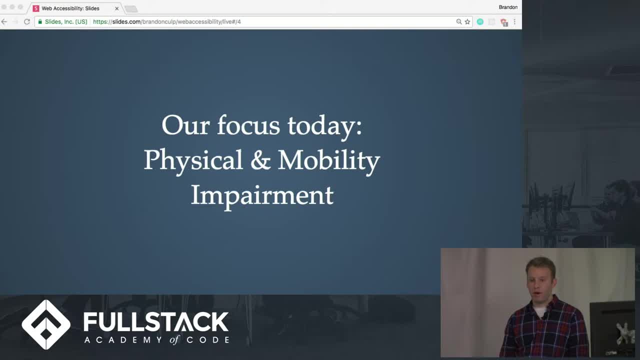 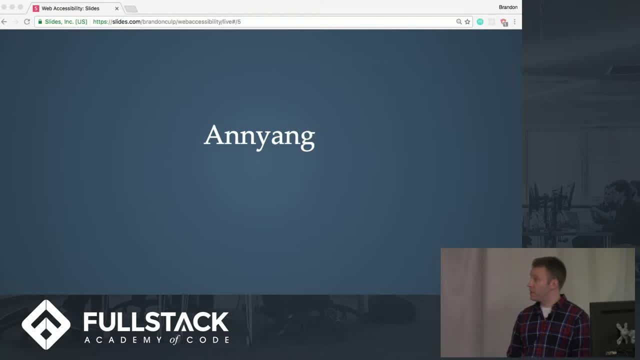 So this is a lightweight library that just utilizes the Google Web Speech API so that you can navigate the site using basically pre-planned commands that you input. So basically, you just have these commands and then they map to function. So whenever the API recognizes, 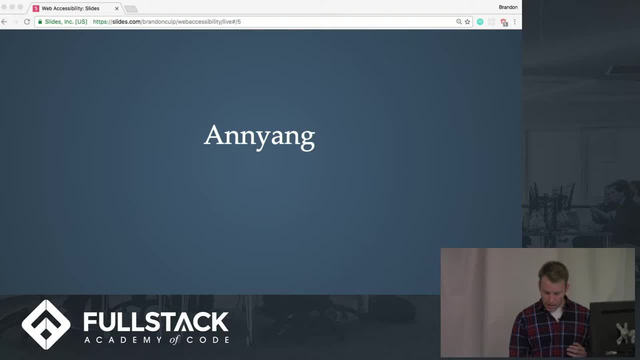 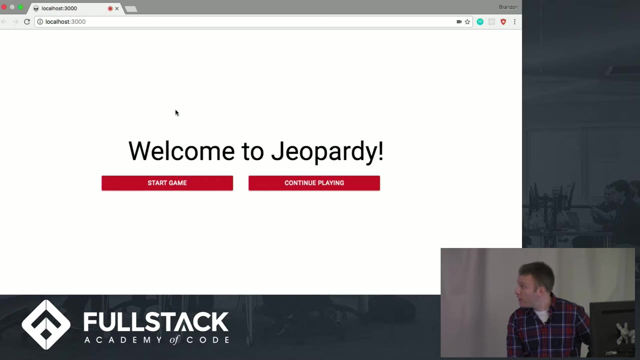 the command, it'll just execute that function. So I recently made a Jeopardy game, as some of you know, for Stack-a-thon, And so I just want to show that real quick. Here is the Jeopardy game. 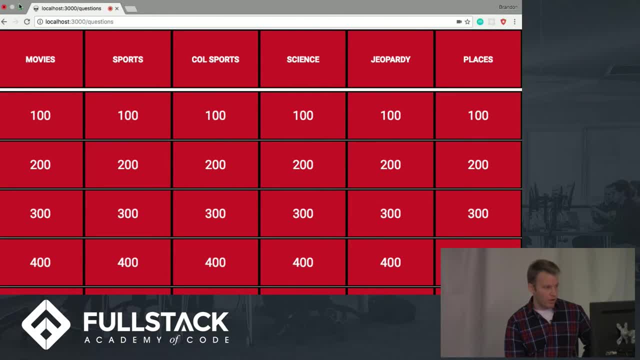 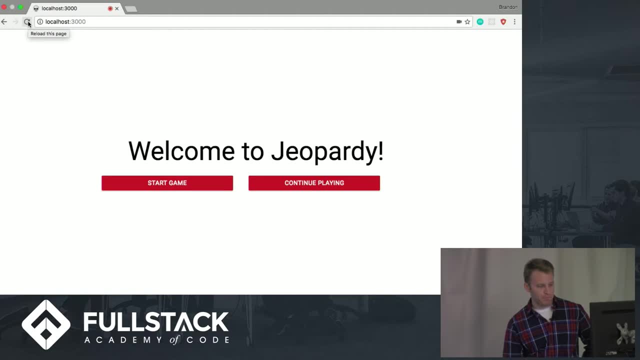 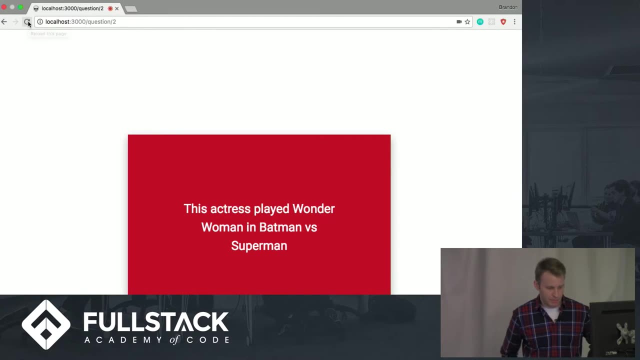 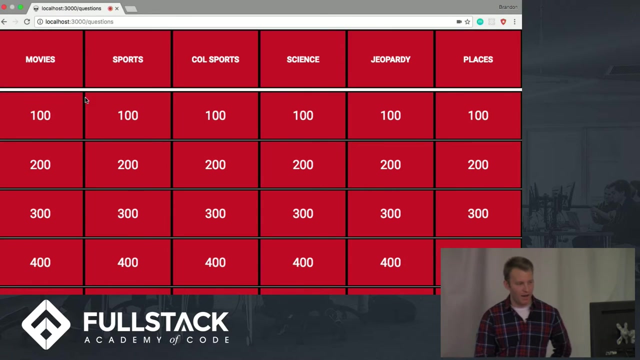 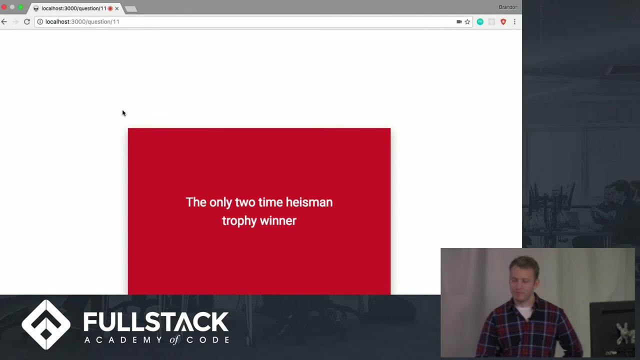 You can start a game, but you can also use your voice. Go back, start game movies 200, Gal Gadot. Who is Gal Gadot? Next question: College sports 400.. Okay, Let's see, I think it's. who is Archie Griffin. 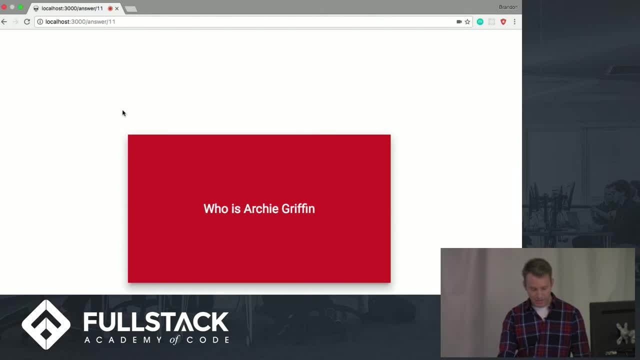 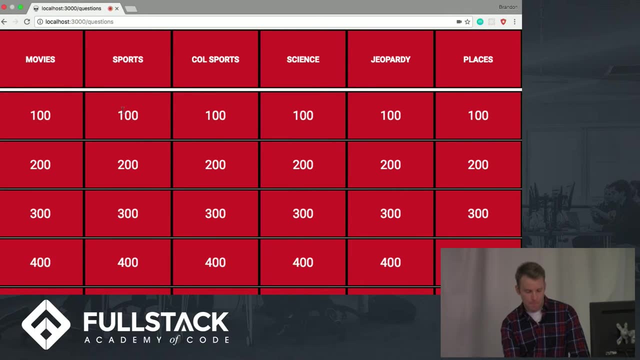 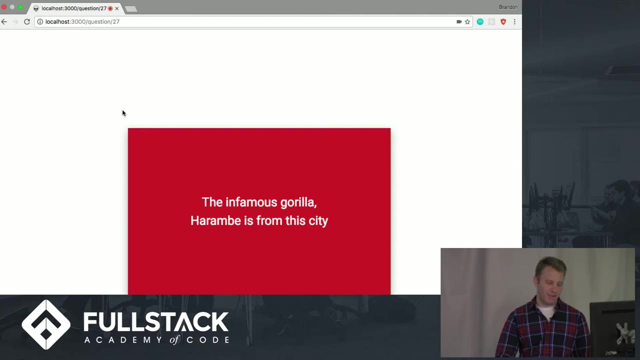 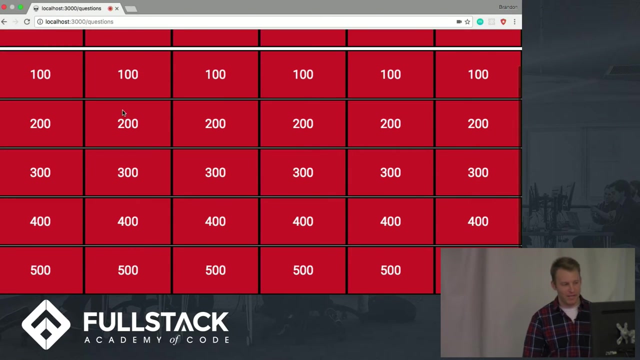 Next question And then finally places 200.. What is Boston? Oh no, that's not right. What is Cincinnati? Next question, Okay, Next question. So that's the basic functionality. Pretty simple. Again, you know, I just have command set up and they're just going to execute, and you know. 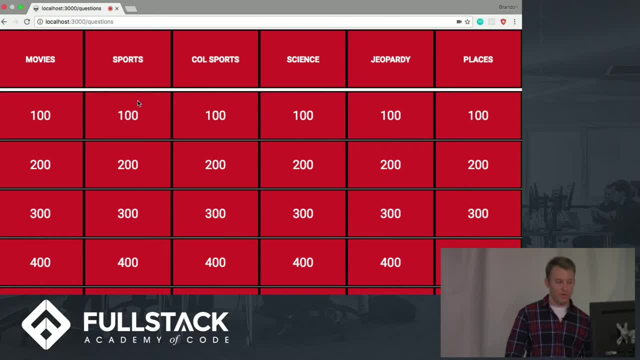 pull up the questions and, as you can see, if you get the question wrong, it'll just sit there and be like you know it's obviously not right, Or for the sticklers for Jeopardy, who you know it has to say who is or what is. 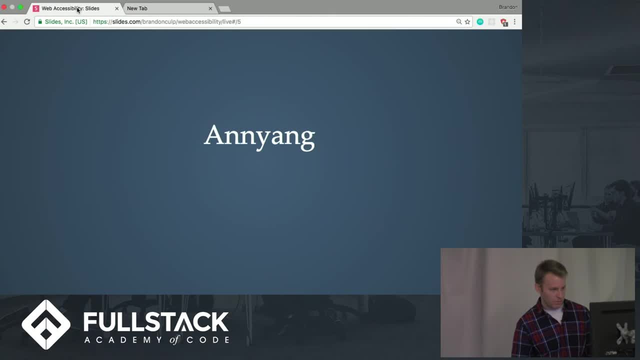 That's in there as well. Okay, Next question: So some additional resources I want to talk to you guys about, for you know you using in your daily life to make things accessible. So there's Alijs, which is basically it will analyze your site and tell you which 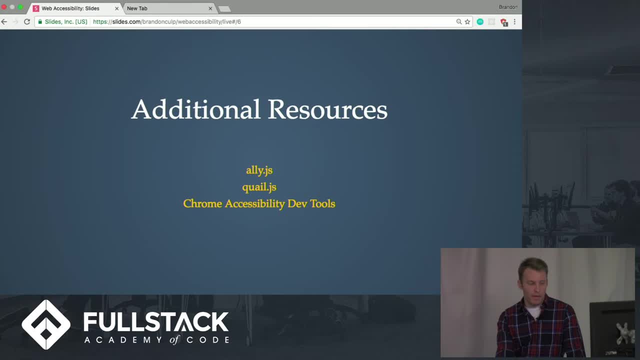 DOM elements can be accessed using a keyboard, and that's, you know. one of the biggest things for people is, you know, moving beyond just the mouse function. Okay, All right, So there's the mouse functionality, And then we also have Quailjs. 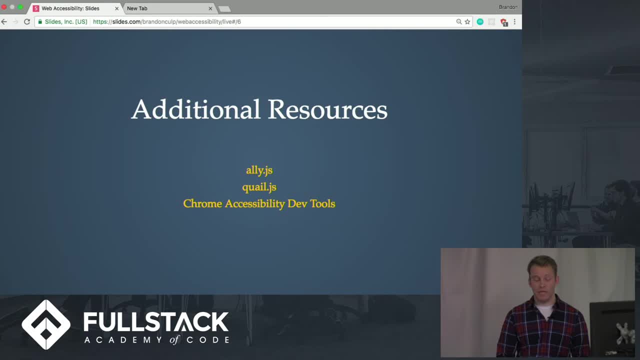 So that's a jQuery plug-in that provides over 200 tests. So, as you're doing your TDD, you can also write tests for accessibility and again, you can, you know, make your own tests. So you know, again, think of your audience and tailor those tests for them. 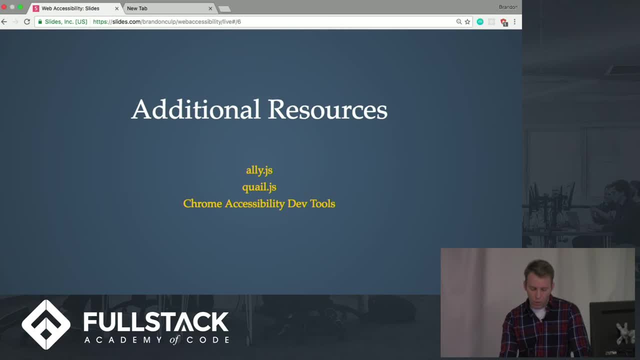 And also something that's cool with that is that actually includes the web content accessibility guidelines, So the version like 1.0 and 2.0. So you'll actually know those guidelines, Okay, And be able to meet those. 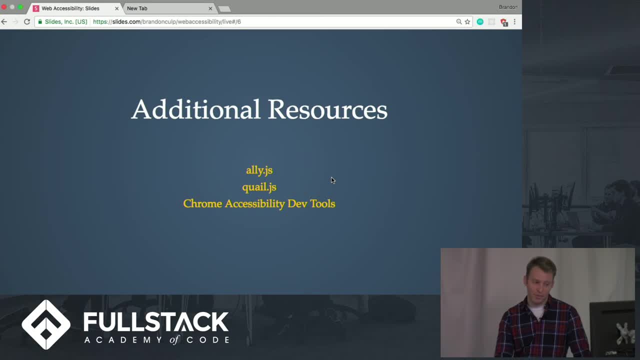 And then, of course, there's a dev tool- Chrome dev tool- for accessibility, So that'll do the basically the checking in live time of your site and tell you right on the page you know, what is accessible and how you can make improvements. 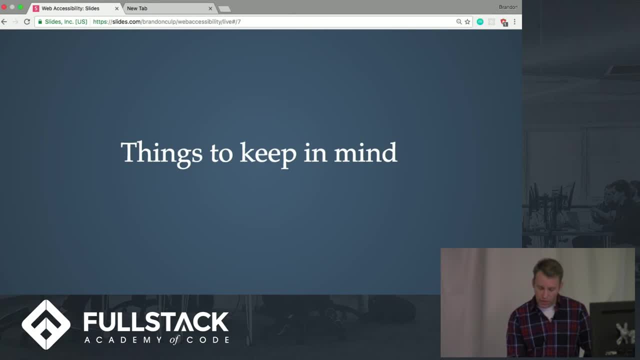 So just to wrap up, some things to keep in mind. So 20% of the population has some kind of disability. so you know, maybe you or I don't have one, But a lot of people do, even if it's just color blindness or something like that. 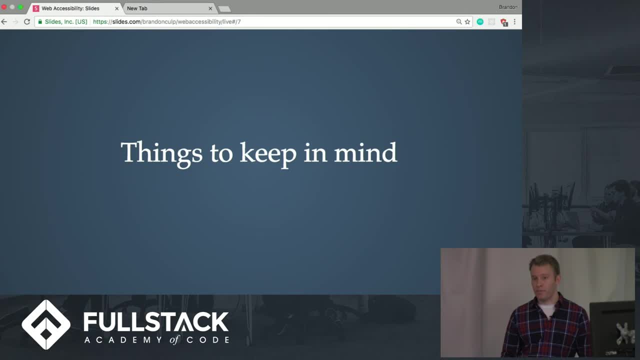 So if you're not designing your website to be accessible for them, you're missing out on a large chunk of the population And also web accessibility benefits a lot of people. So kind of like I just showed you you know a library like that is pretty cool and you. 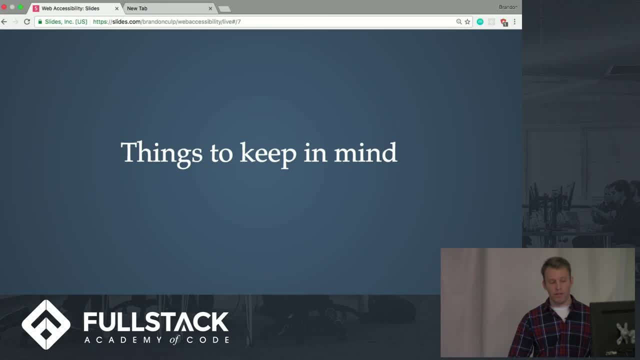 know, doesn't have to be just for someone with a disability. You know, one of the things with accessibility is making your site flexible for multiple people in multiple situations. So even if it's just, you know, someone that has a slow internet connection, you know.